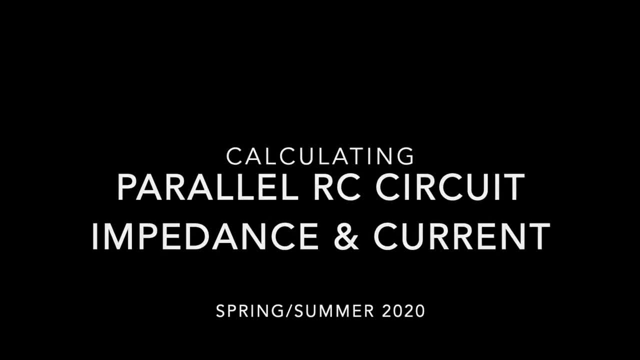 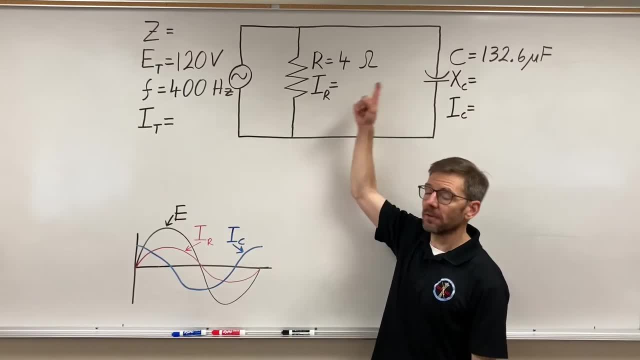 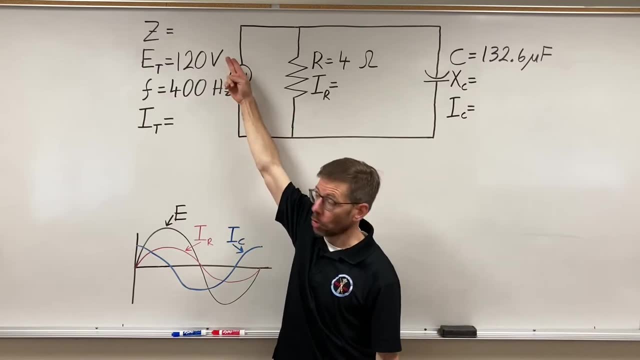 Okay, here we are with a parallel RC circuit, Resistive, capacitive RC parallel, And we're going to try and find impedance, total circuit opposition and total current. We could do it a couple of ways to get the impedance. We're going to start off with the formula. 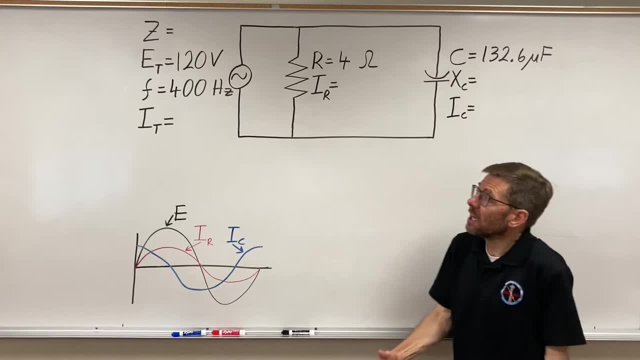 version this time, And what I need to do is it's kind of that product sum and Pythagoras mashup in the formula of my resistance and my Xc, my capacitive reactance. So I need to calculate that first. Quick reminder on how to do that Long formula. we can do it. 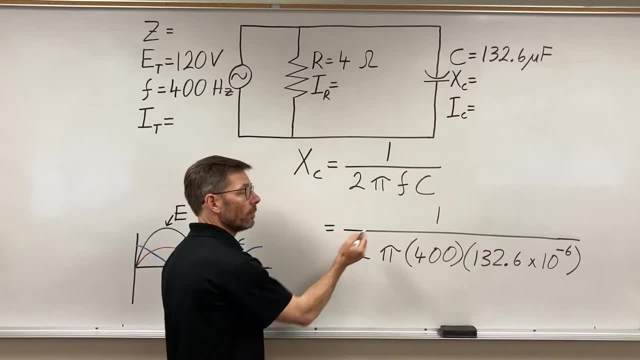 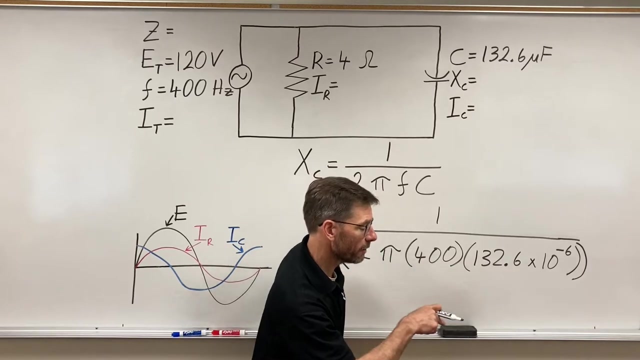 Now we want to make sure again that when we're dividing by a quantity we put that whole quantity in parentheses. So 1 divided by parentheses, 2, pi double. check your frequency. Here we've got 400 hertz times 132.6,. second function: double. 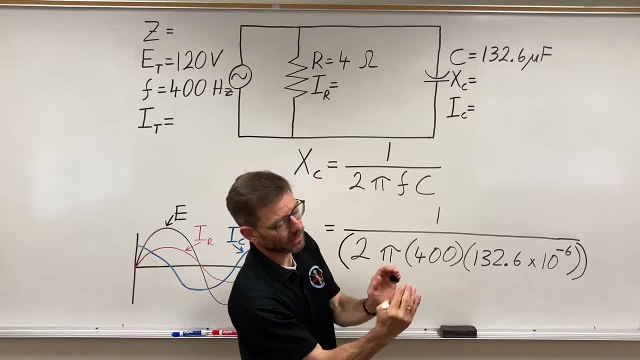 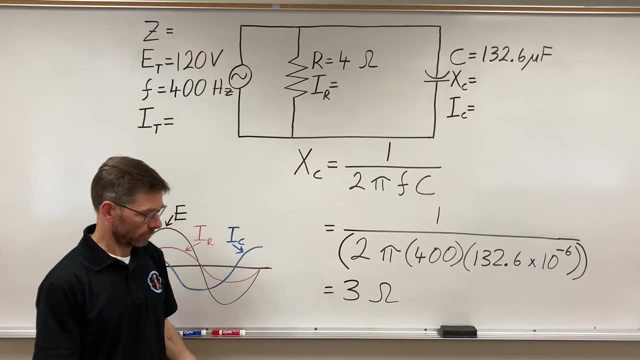 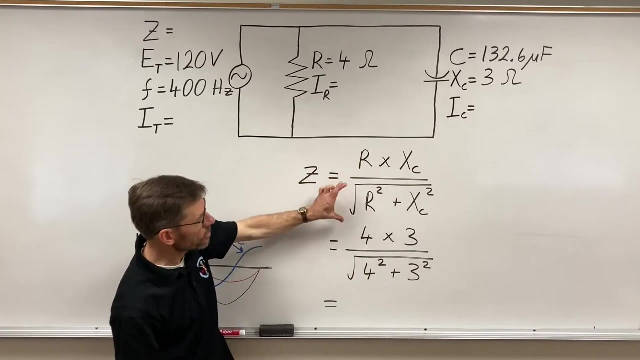 E minus 6, the little negative with the parentheses around it, And what do we come up with? 3 over 0.. Here's that mashup formula. It looks a little like product sum, but also like Pythagoras, Because the objective here, as we remember with our parallel circuit rules, is the total. 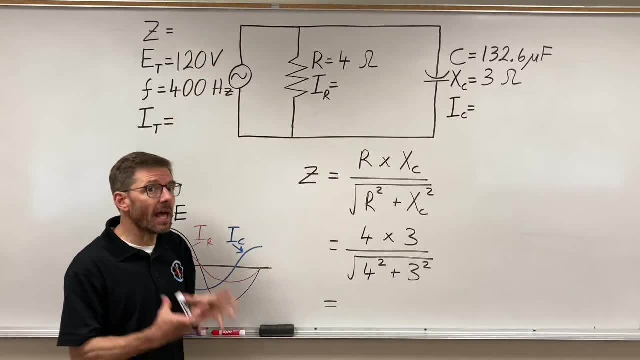 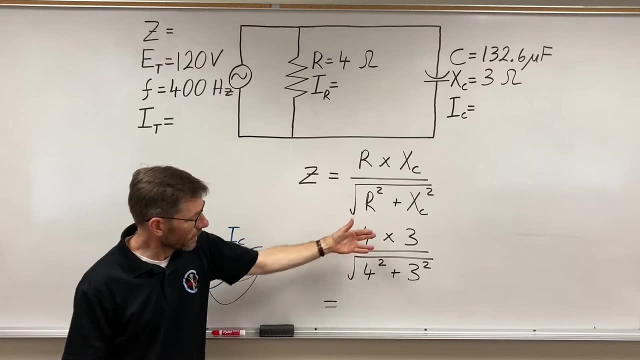 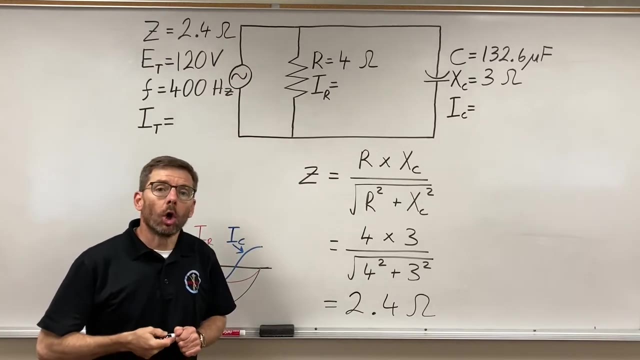 circuit, opposition is going to be less than either one of these in an RC circuit. So as we plug that in, what do we get? 2.4 ohms And sure enough, that's less than either one of those, Less than 3,, less than. 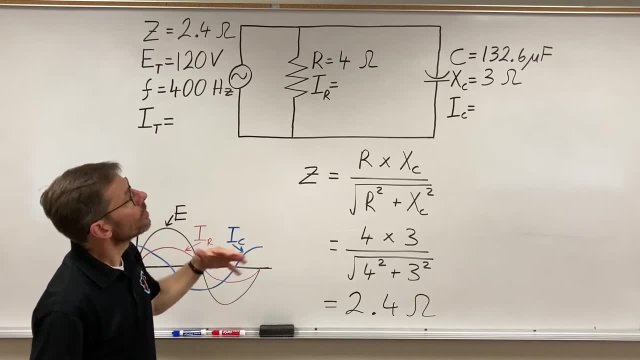 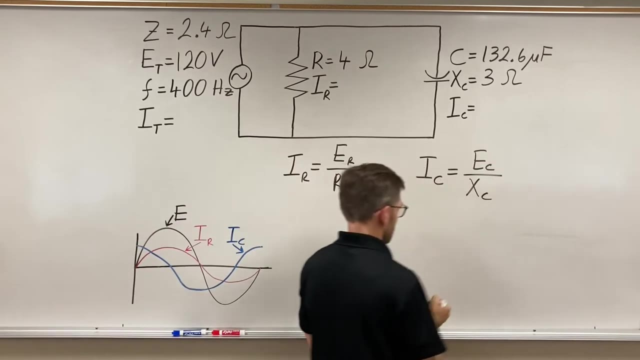 4, 2.4.. Excuse me. So now we're going to find out our currents vectorially, add them and then do Ohm's law just to double check our impedance. And the formulas we'll use are Ohm's law. 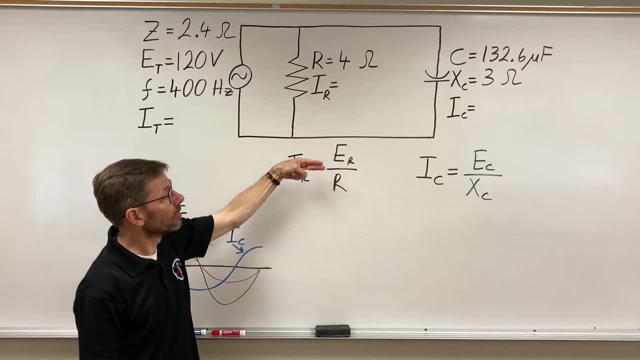 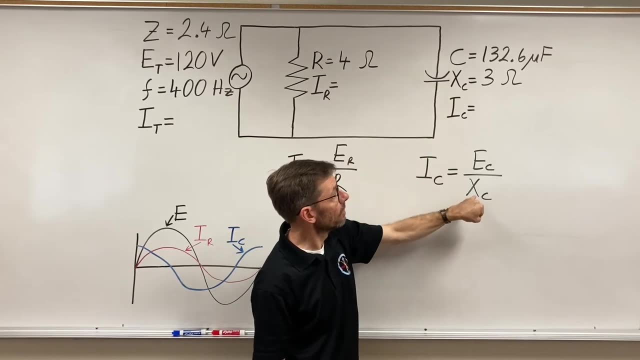 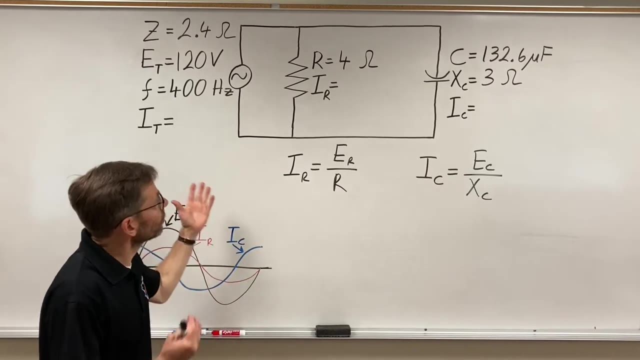 The current on the resistor uses the voltage and the resistance the values on the resistor. Likewise for the capacitor: the voltage here and its Ohmic value. Now remember what do I like to do when I draw parallel circuits? I didn't do it. I probably should have done. 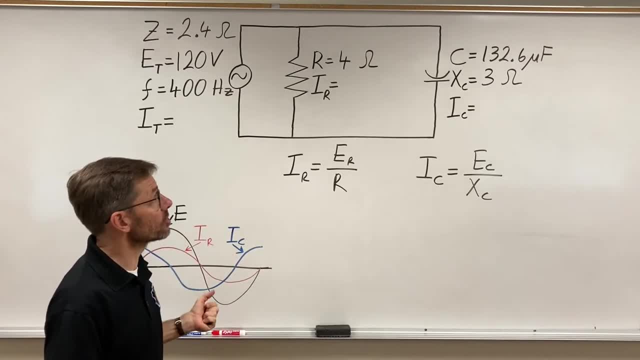 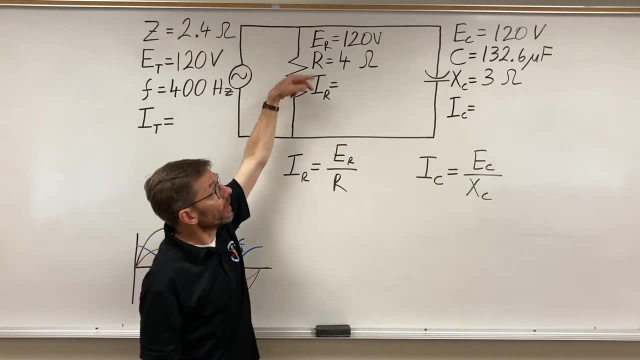 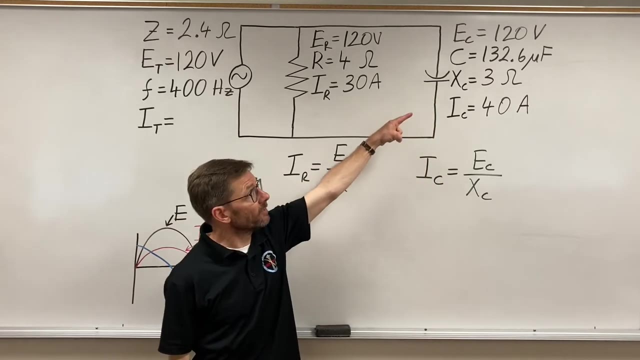 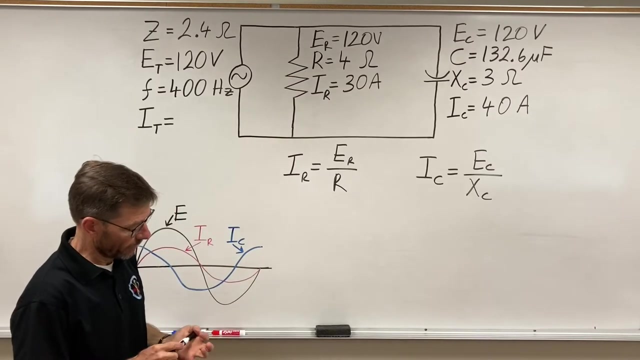 it already is. draw my voltage on both branches And once I have those written up there, it's pretty intuitive. Volts and Ohms, And what do we get? 120 divided by 3 is 40 amps. 120 divided by 4 is 30 amps flowing. Now those amps are not. 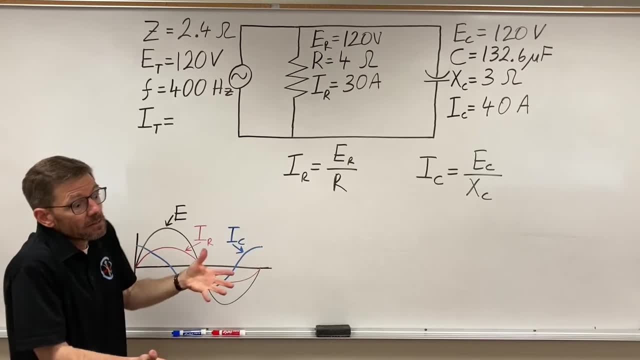 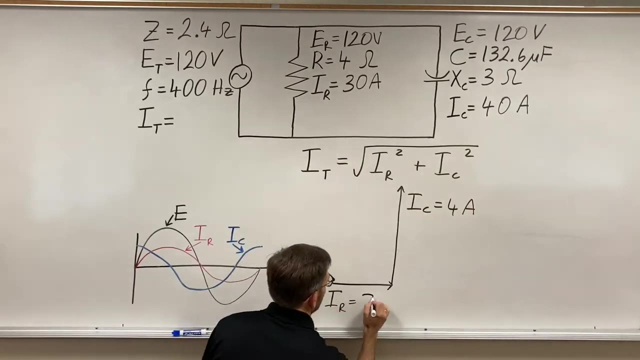 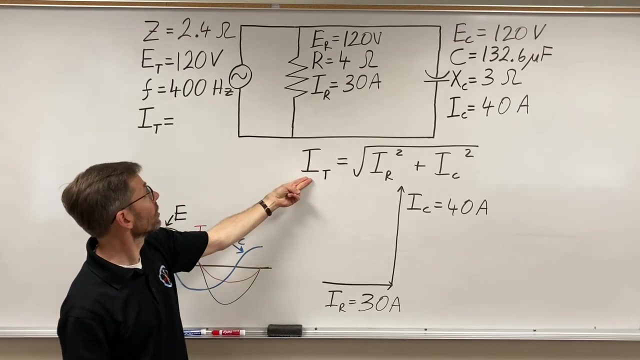 in phase with each other, so they don't just add simple arithmetically. So what we do is we vector them 90 degrees apart. So I drew the formula which is Pythagorean Theorem, and that'll yield our total current. 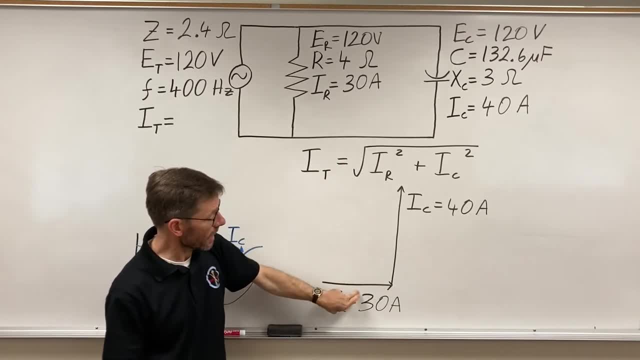 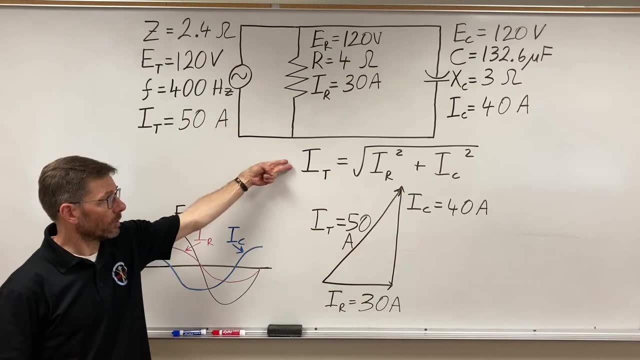 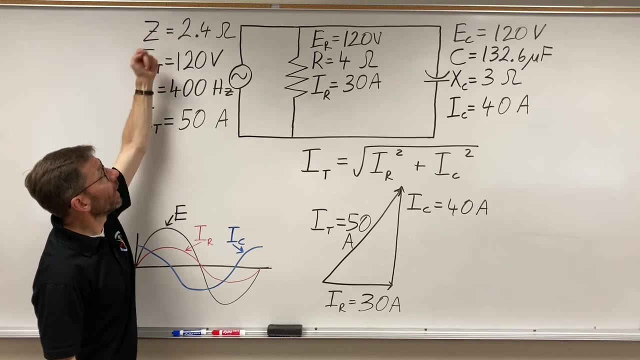 We can also look at them as vectors, because that's what Pythagorean is: a squared plus b squared is c squared And 50 amps, whether we use the formula or, let's confirm, 120 divided by 2.4.. 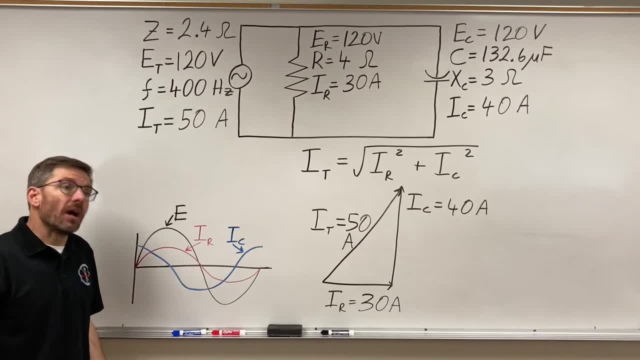 50 amps. Now, these 50 amps are not necessarily gonna be in-phase with a voltage or 90 degrees out. Remember, they're a mix between the two. They'll combine and they'll kind of pull: The resistor wants to pull it in-phase, the capacitor 90 degrees out. so they're going to meet somewhere. 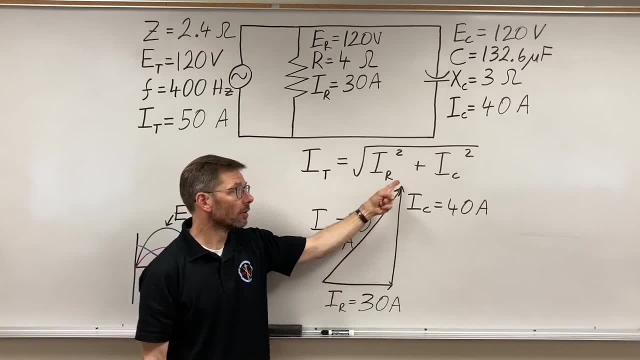 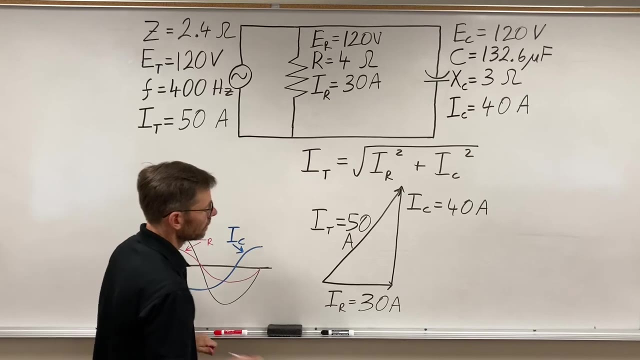 in the middle And because there are more reactive mains and there are quantum fields and there are more sources of energy- active amps- than there are resistive- that angle is greater than 45. It's more capacitive than it is resistive. Could we figure out angle theta from here? Yes, Angle theta, the cosine of angle theta.